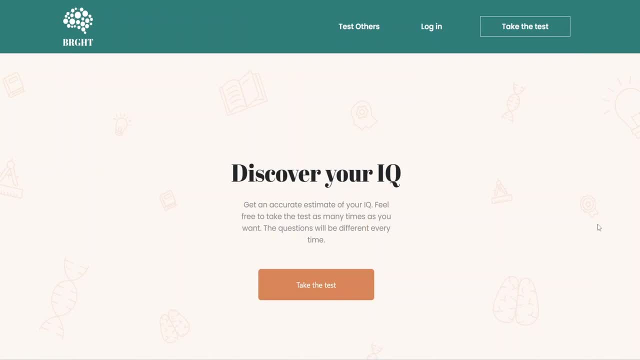 Hi there, welcome to Puzzles and Solutions. Today I will go through the full Brightorg 40-minute IQ test. For this video I will not go through the puzzles live. Instead, I've already completed the test and I will explain the puzzles now, after solving it. 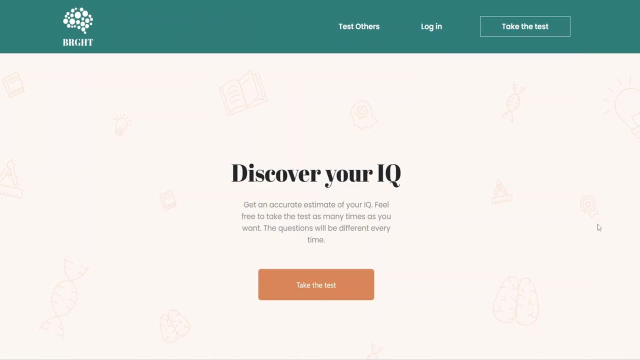 I think the IQ test is very well designed and the puzzles are fun. A bad thing about this site is that the full 40-minute test is not free. You have to pay to see the score after completing the 40 minute test. However, there is also a half 20-minute test that is free. Feel free to pause. 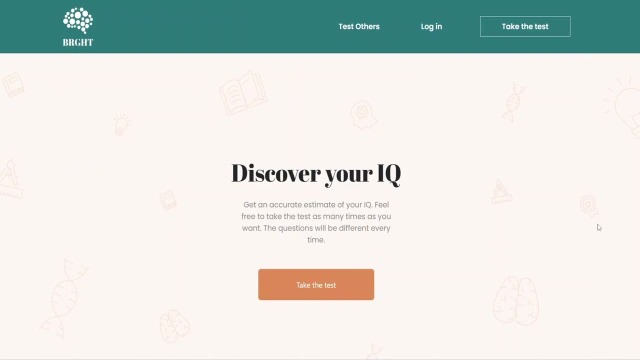 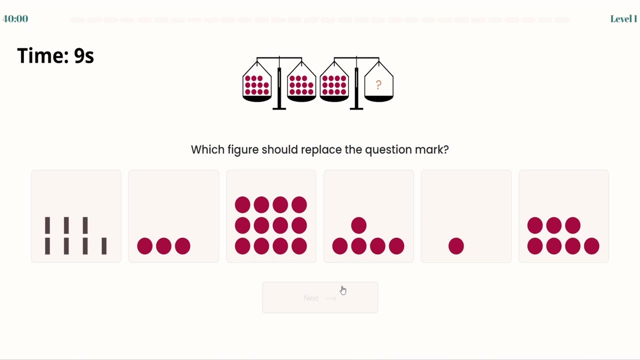 at each puzzle and give them a shot yourself. Let's start. Which figure should replace the question mark? When I took the test, I answered this question in nine seconds. You can see the time in the top left corner of each puzzle To solve this puzzle. we can see that in the first scale we have 11 red circles. 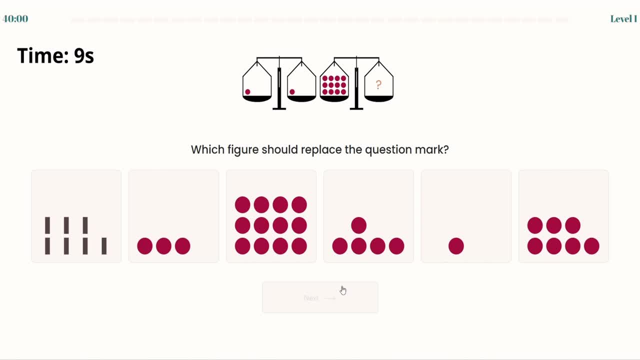 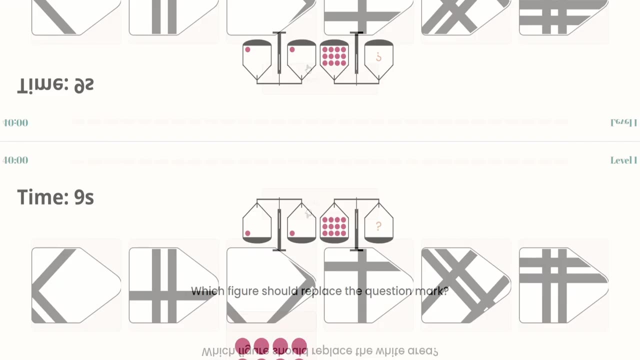 on each side, so one red circle on the left is equivalent to one red circle on the right. The answer should have as many red circles as the left side of the second scale, so 12 red circles. Answer 3 is correct. Which figure should replace the white area? 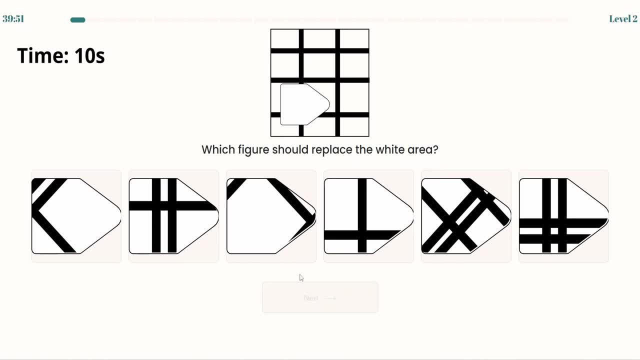 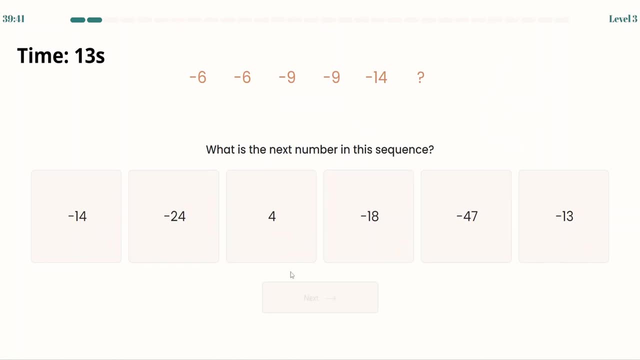 Here I just mentally visualize a continuation of these black lines giving this black cross identical to answer 4.. Answer 4 is correct. What is the next number in this sequence? This one is pretty obvious: Minus 6 minus 6, minus 9 minus 9, minus 14 minus 14.. 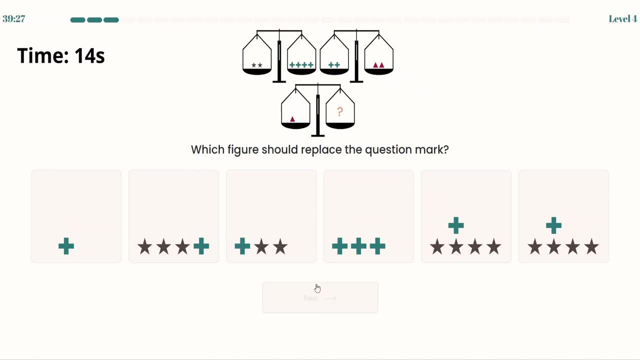 Answer 1 is correct. Which figure should replace the question mark? In the second scale we see that a plus sign is the same weight as a triangle, And in the third scale we have a triangle on the left side. so one possible answer is a plus sign. Answer 1 is a plus sign. Answer 1 is correct. 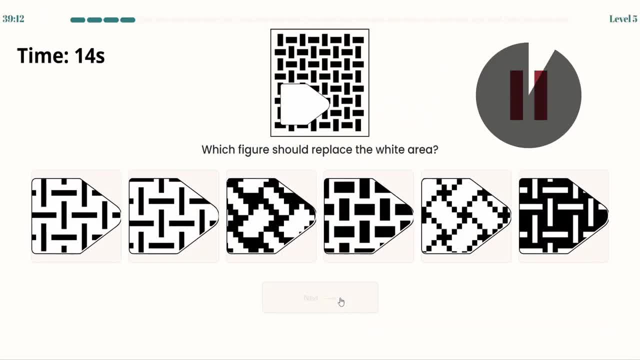 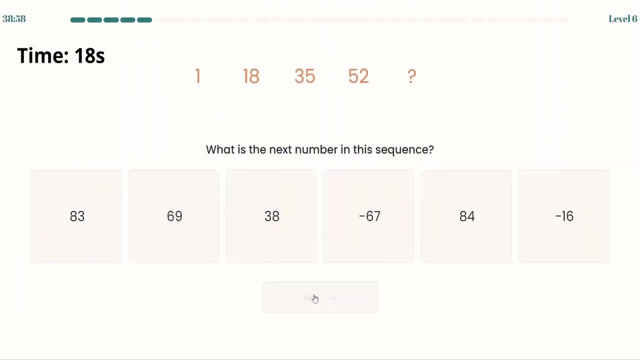 Which figure should replace the white area In the image? we have these black rectangles with widths and heights. that matches answer 4.. Answer 4 is correct. What is the next number in the sequence 1?, 18?, 35?, 52?? Answer 2 is correct. which sequence should replace the question mark? Who is on the correct lineذاbooks or the right was? Excuse me, 1? 18? 35, 52? Here we just add 17 to generate the next number. So 1 plus 17 is 18, 18 plus 17 is 35, 35 plus 17 is 52 and 52 plus 17 is 69.. Answer 2 is correct. Which sequence should replace the question mark? If a ciudad is a square and observation, öffentlichاتqspotter ملتدنية doesn't come up with the direction of 1 and 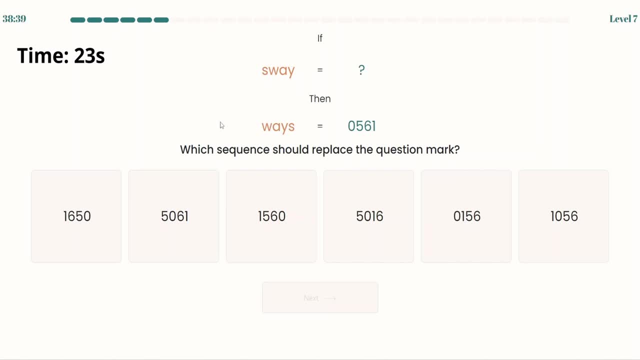 equals question mark, then ways equals 0, 5, 6, 1.. For this puzzle I realized that to convert ways into sway, all you have to do is take the last character, s, and move it in front, and you could do the same with the sequence. so you take the 1 at the end of 0, 5, 6, 1 and put it in front to get. 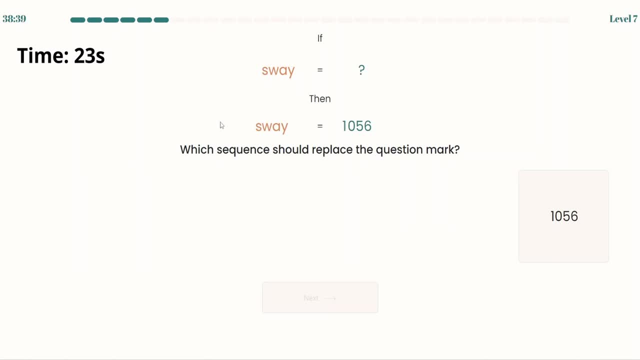 1, 0, 5, 6.. Answer 6 is correct. Which 3 shapes can be combined together to create the figure on the left? I just imagine that I take different shapes and try to fit them together, so shape 3 fits on. 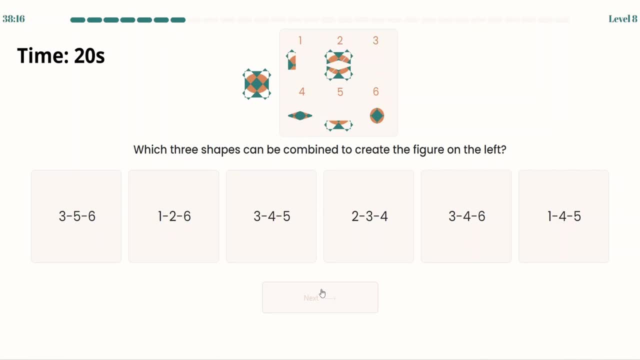 the left side of shape 2 and shape 4 fits in the middle of these two shapes: 2, 3, 4.. Answer 4 is correct. Which number should replace the question mark? We multiply the two numbers on top and divide by the number. 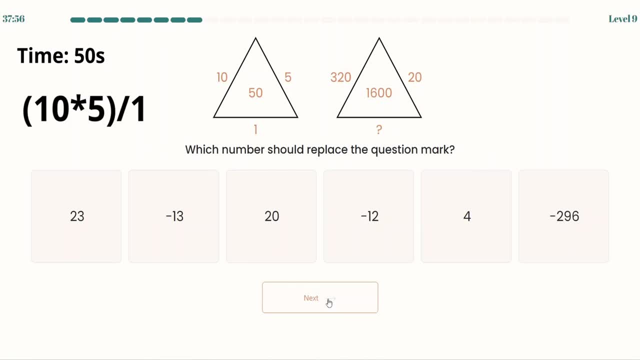 under. So for the first triangle we have 10 times 5 divided by 1, which of course also is 50. And for the second triangle we have 320 times 20, 6400 and divided by 4 is 1600.. Answer 5 is correct. 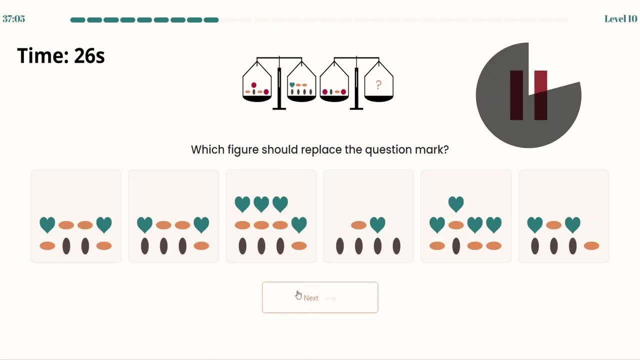 Which figure should replace the question mark? Here I realized that the left side of the first scale can easily be converted into the left side of the second scale. All we have to do is eliminate one of these yellow ovals. This means that the right side of the first scale is equivalent to the answer. It matches answer 4.. Answer 4 is correct. 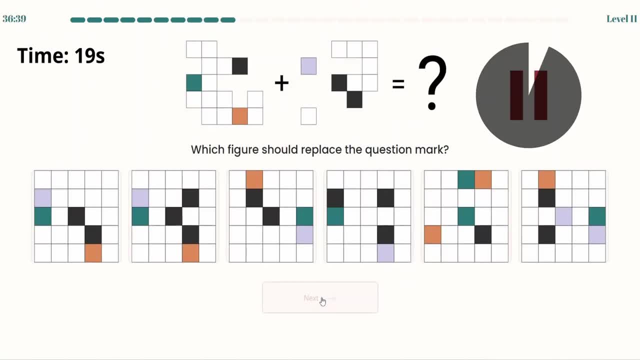 Which figure should replace the question mark? I think the first one. Answer 4 is correct. Which figure should replace the question mark? I think the first one. the easiest way to explain this puzzle is by doing a visual proof, So by just adding the two shapes. 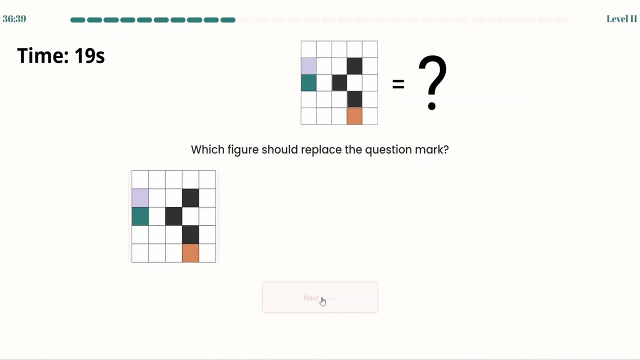 together we see that it matches answer 2.. Answer 2 is correct. What is the next number in this sequence? 8, 2, 1 over 3, 1 over 24, question mark: If we take 8 divided by 4, we get 2.. 2 divided by. 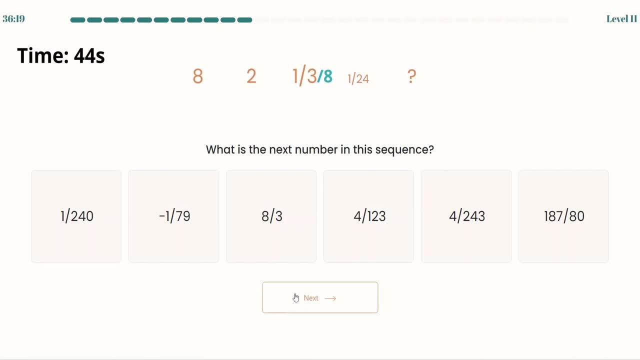 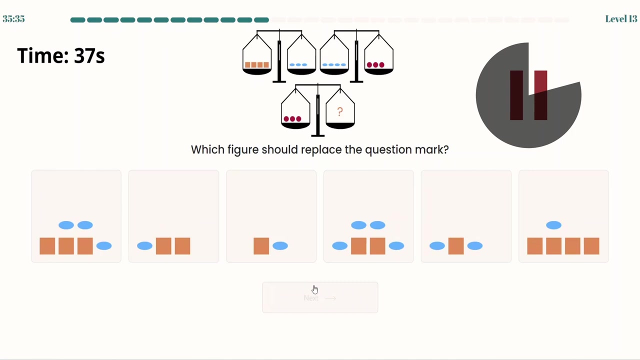 6, we get 1 over 3.. 1 over 3 divided by 8, we get 1 over 24.. 1 over 24 divided by 10, we get 1 over 240.. Answer 1 is correct. Which figure should replace the question mark? So for this puzzle. 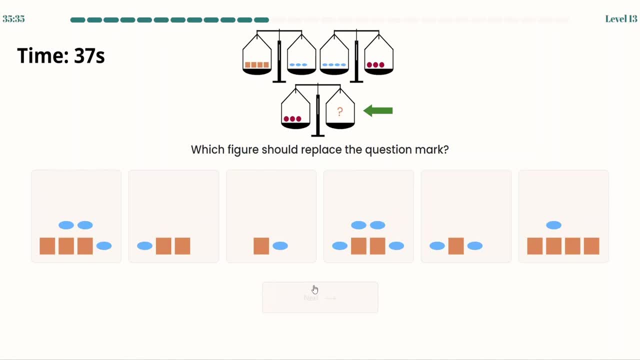 I'm going to focus. on the left side of the third scale, We have three red circles and, based on the second scale, we can convert it into four blue circles. So for this puzzle I'm going to focus, also based on the first scale, we can convert three of these blue ovals into four yellow. 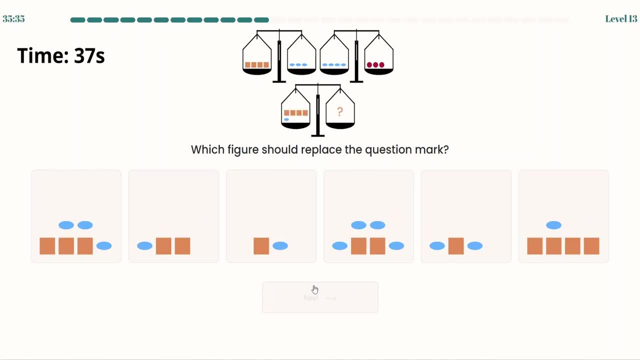 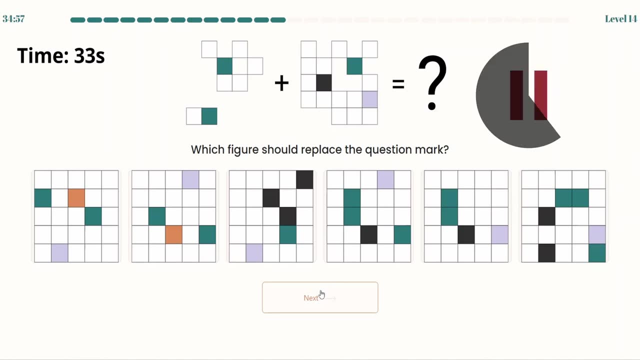 squares. This left side is now equivalent to answer 6.. Answer 6 is correct. Which figure should replace the question mark? Again, we have one of these visual puzzles. I will just add together the two images and we see that it's identical to answer 4.. Answer 4 is correct. 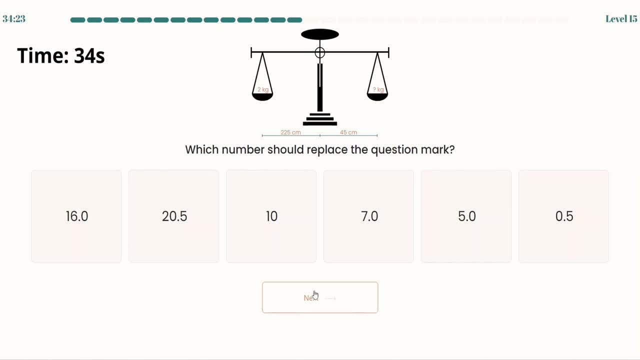 Which figure should replace the question mark? Answer 4 is correct. Which number should replace the question mark? On the left side we have 2 times 225, giving 450.. We should have the same on the right side Question mark. times 45 should be equal to 450.. 10 times 45 is 450.. Answer 3: 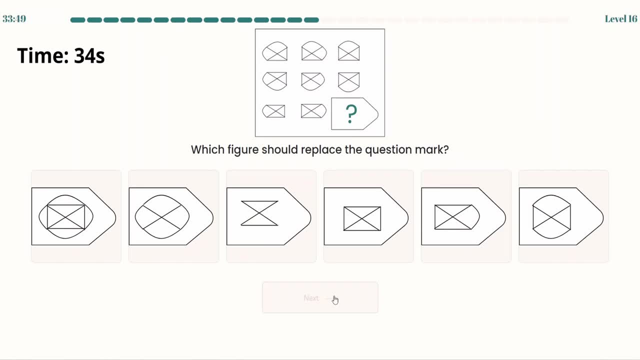 is correct. Which figure should replace the question mark? Answer 3 is correct. Answer 4 is correct. Which figure should replace the question mark? Answer 3 is correct. Answer 5 is correct. Answer 6 is correct. Answer 7 is correct. Answer 9 is correct. 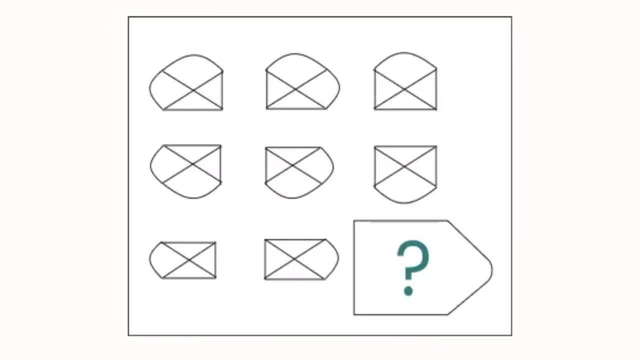 So here we see that every image in each row is identical, except for this left side in the first column and this right side in the second column. So, based on the third row, without this thing on the left side or the right side, we just expect this rectangle with a cross in the middle. 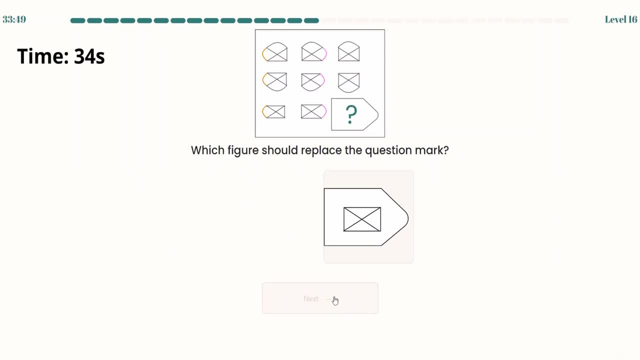 Matching answer 4.. Answer 4 is correct. Which tree shapes can be combined to create the figure on the left? Shape 2 fits on top of shape 1, and shape 3 can be placed in the middle of shape 1 and 2.. 1,, 2,, 3,. answer 2 is correct. Which number should replace the question mark? 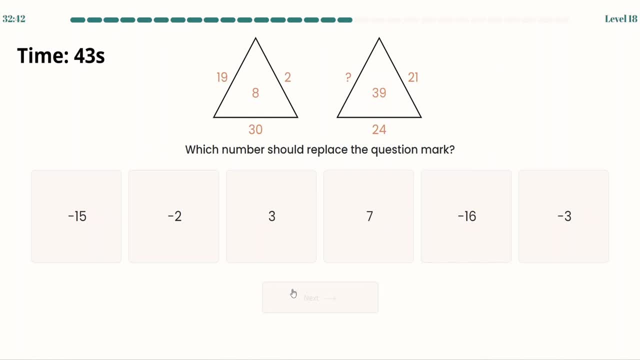 In the first triangle to get the number inside 8, we can look at the numbers outside and take 19 times 2 minus 30. So multiplying the numbers on top minus the number on the bottom, And looking at the second triangle, we have a question mark. times 21 minus 24 equals 39. The only integer 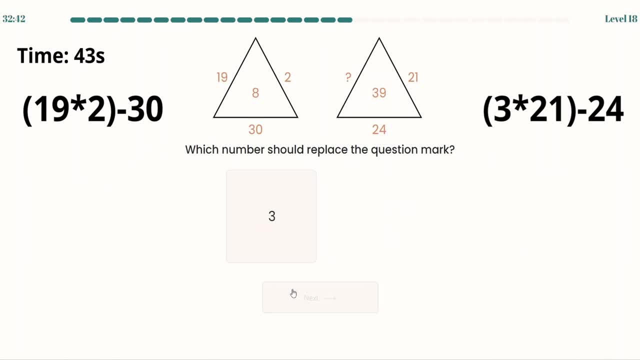 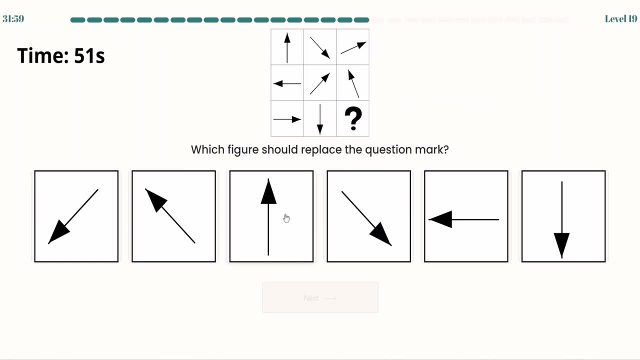 that fits this equation is 3.. Answer 3 is correct. Which figure should replace the question mark? So this puzzle gave me flashbacks to vector addition. I'll show you what I mean, So I will colour each column in a different colour: red, green, blue. 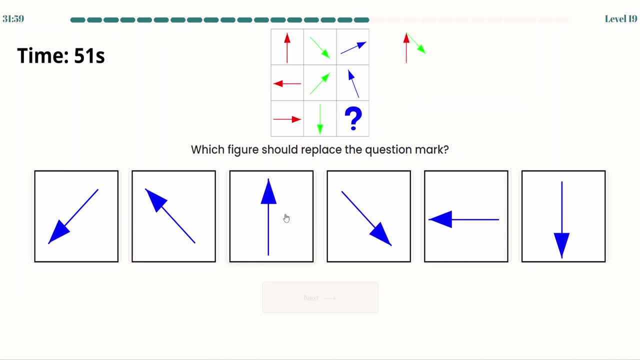 If we take the red arrow and then attach the green arrow at the tip of the red arrow, then the blue arrow will go from the start of the red arrow to the end of the green arrow and a tiny bit further. This is the concept of vector addition, except that the blue arrow should point the end. 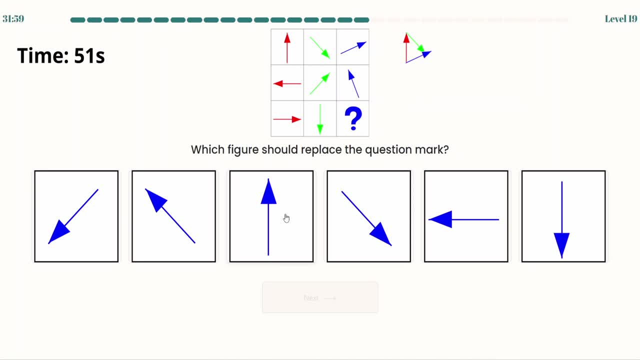 of the green arrow. This also works for the second row. So red arrow, green arrow and a blue arrow. that's a bit longer. So to solve this puzzle we have to look at the third row. So we take the red arrow and attach the start of the green arrow to the end of the red arrow. 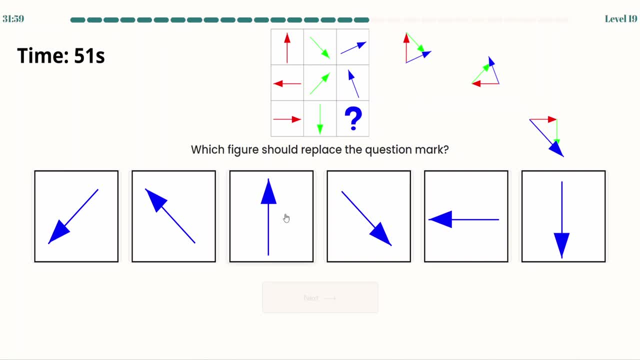 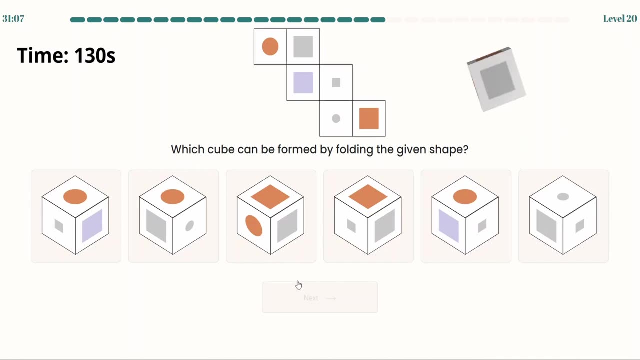 The blue arrow should then point from the start of the red arrow to the end of the green arrow and a bit further. This matches answer 4, answer 4 is correct. Which cube can be formed by folding the given shape? My first plan was to explain this puzzle in words, but I realized that it's very hard. 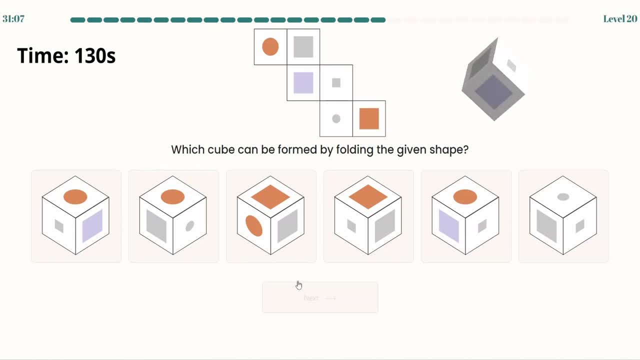 so instead, I created this 3D model of the cube. By rotating this 3D cube to a specific side, we see that it matches answer 3,. answer 3 is correct. Oh, by the way, When I did the test, this was my first incorrect answer. 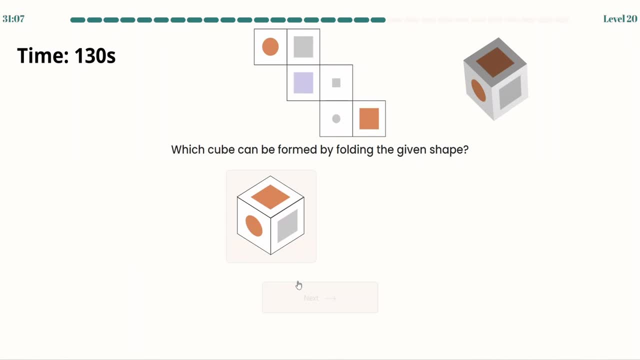 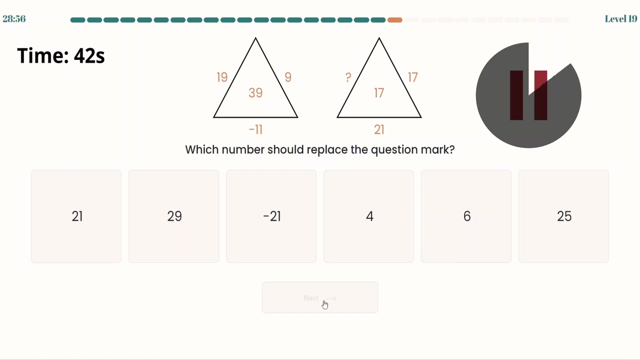 I spent around 2 minutes on the puzzle and then I realized that I was spending a lot of time on this puzzle and I didn't really have a good idea what the correct answer was, so I just guessed, And I guessed wrong. Which number should replace the question mark? 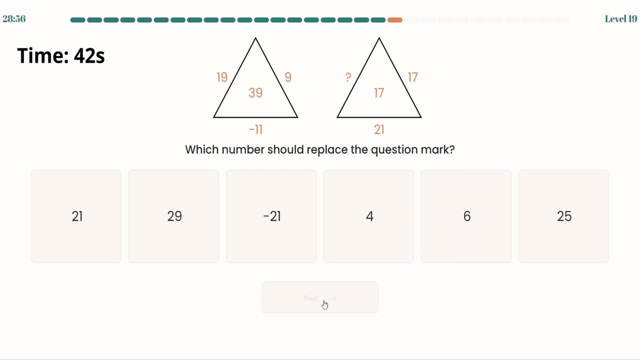 So I got flashbacks to the previous one of these puzzles where we multiplied the two numbers on top Minus the number under to get the number in the middle of the triangle. This puzzle is pretty much the same, except that we add the two numbers on top. 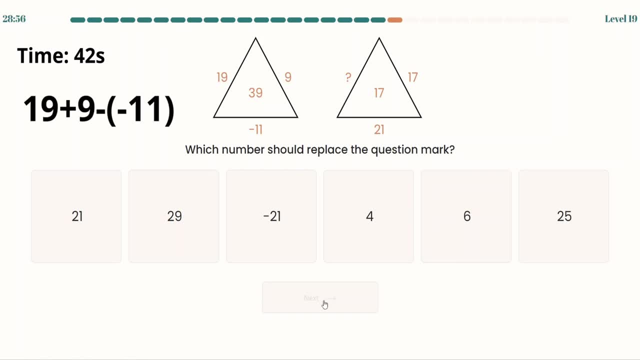 So in the first triangle it's 19 plus 9 minus minus 11.. This is equal to 39.. For the second triangle we have a question mark: plus 17 minus 21 is 17.. So of course we need 21 minus 21 to count. 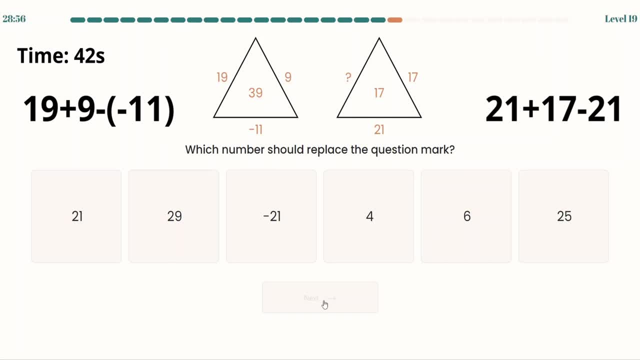 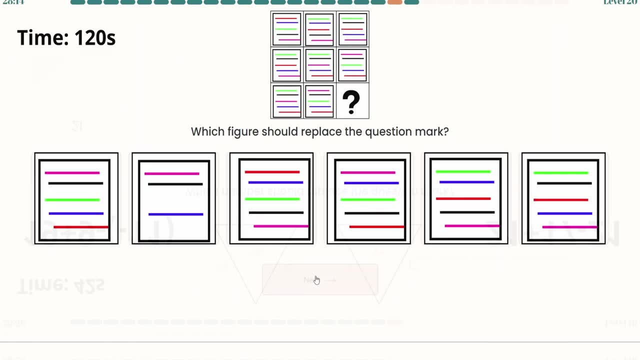 So we have a question mark: plus 17 minus 21 is 17. So of course we need 21 minus 21 to count. We cancel out to get that 17 equals 17. So the answer should be 21.. Answer 1 is correct. 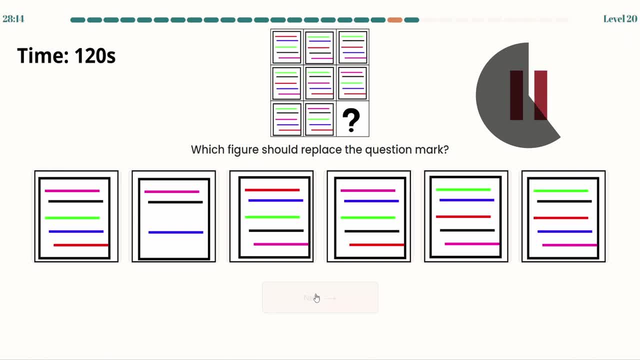 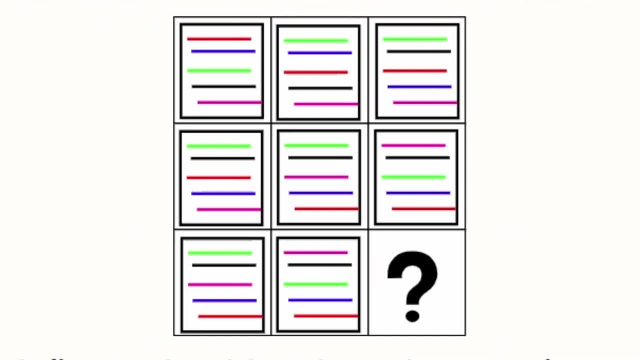 Which figure should replace the question mark? So, looking at the first row, going from the first image to the second, we swap the position of the first and the third line, Going from the second to the third image, we swap the position of the second and the. 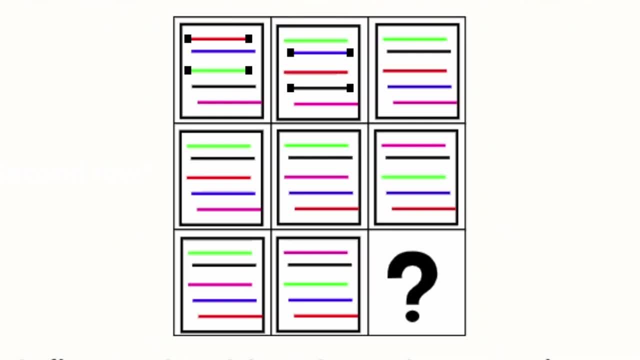 fourth line In the second column. we go from the first image to the second by swapping the position of the third and the fifth line, And then from the second to the third. we swap the position of the first and the third line In the third row, going from the first to the second image. we swap the position of 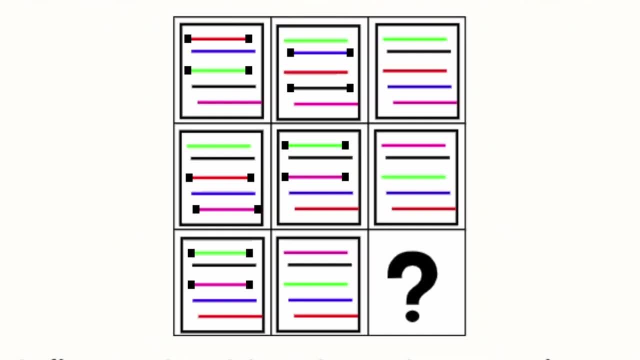 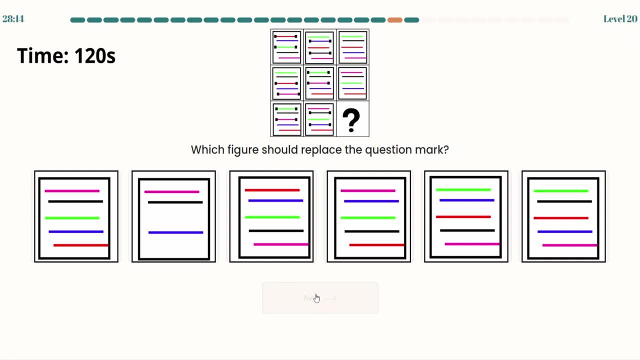 the first and the third line. So, to go from the second image to the answer, I expect that we swap the position of the second and the fourth line: Purple, blue, green, black, red. Answer 4 is correct. Answer 4 is correct. 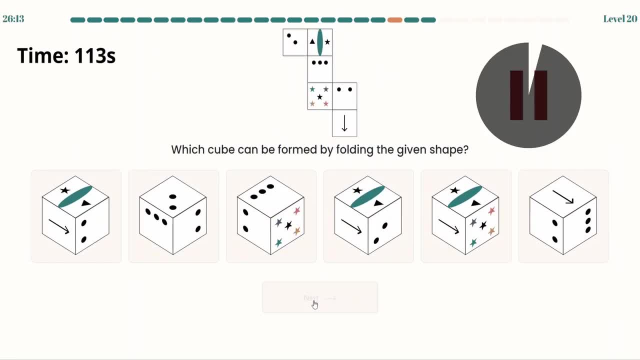 Which cube can be formed by folding the given shape, Another one of these cube folding vessels, Rotating the 3D model to a specific side. we see that it matches answer 4.. Answer 4 is correct. What is the next number in this sequence? 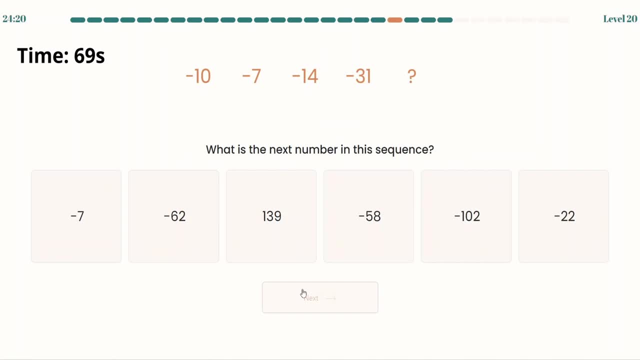 Minus 10,, minus 7,, minus 14,, minus 31? Question mark: Answer 4 is correct. Answer 5 is correct. The pattern of this puzzle was actually quite easy: To go from minus 10 to minus 7, we add 3.. 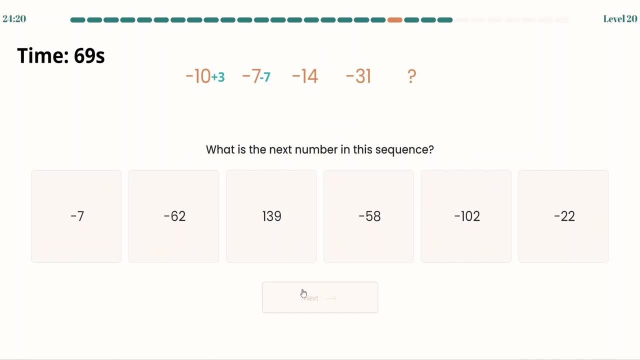 And to go from minus 7 to minus 14,, we subtract 7.. And to go from minus 14 to minus 31, we subtract 17.. And finally, to go from minus 31 to the answer, we subtract 27.. 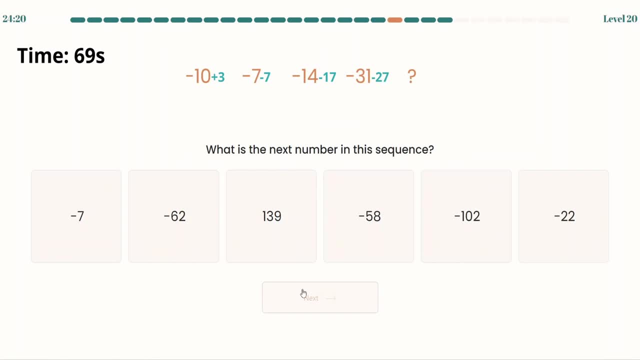 So the amount we add or subtract decreases by 10. For each number we go towards the right: Minus 31,, minus 27, is minus 58. Answer 4 is correct, Answer 5 is correct, and so on. 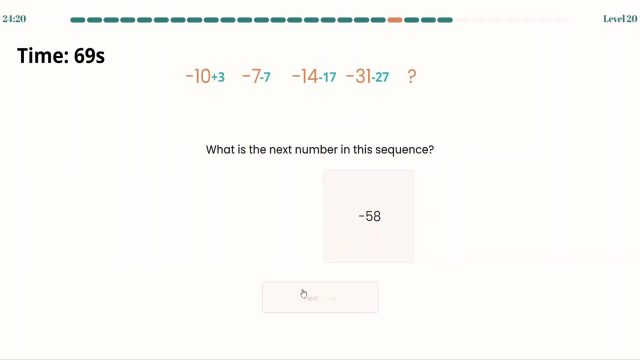 Which figure should replace the question mark? This was a pretty hard situation to solve by only only note how many points there were. The way to solve it is by first, by looking at the first scale and eliminating the 4 stars on each side. כל foundation and除 perspective. 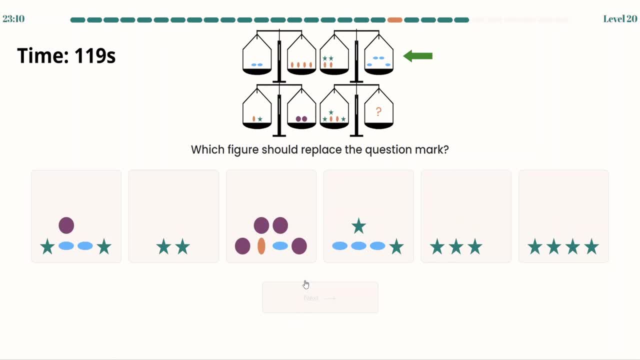 and then we can convert two of the blue ovals on the right side into four yellow ovals, and this allows us to delete the two yellow ovals on the left side against two yellow ovals on the right side. By dividing both sides by two, we get that one star equals one blue oval plus one yellow. 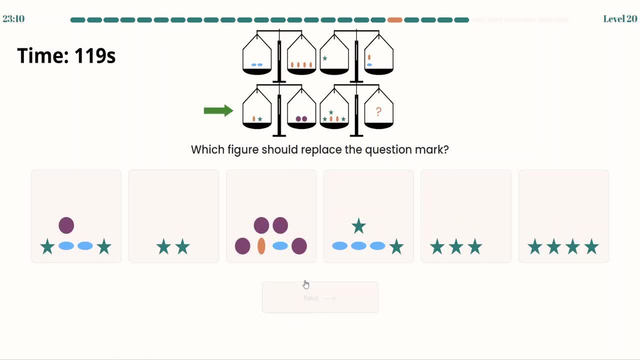 oval. Looking at the third scale, we see that one yellow oval plus one star equals two purple dots. Looking at the fourth scale, on the left side, we can convert two of the stars plus two of the yellow ovals into four purple dots. Based on the second scale, we can convert the remaining star. 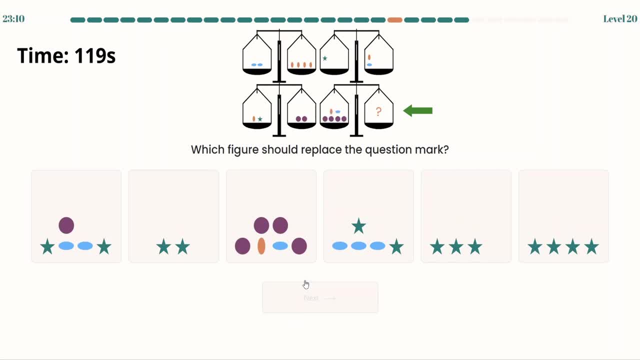 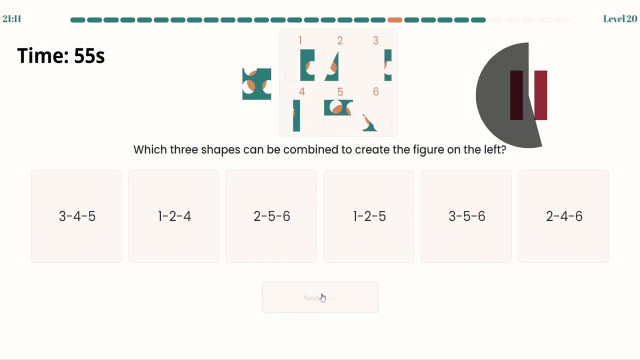 on the left side of the fourth scale into one yellow oval and one blue oval. The left side of the fourth scale is now equivalent to answer three. Answer three is correct. Which three shapes can be combined to create the figure on the left? Shape four fits on the left side of shape three and shape five fits on the left side of shape. 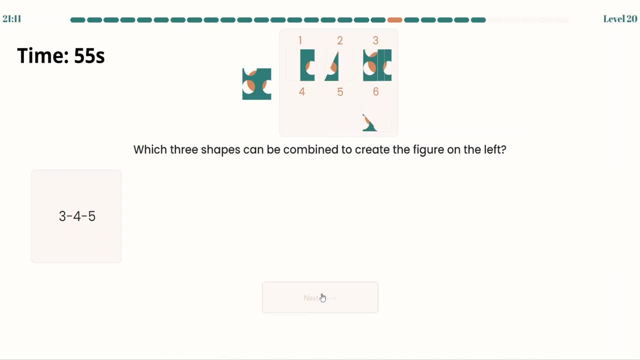 four, Three, four, five. Answer: one is correct. What is the next number in this sequence? Five, twelve, two, sixteen, twenty three, twenty three over six, ninety two over three. question mark: Five plus seven is twelve. Twelve divided by six is two. Two times eight is sixteen. Sixteen plus seven is twenty-three. 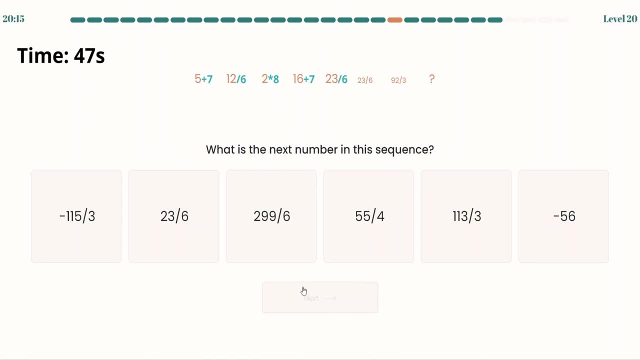 Twenty-three divided by six is twenty-three over six. Twenty-three over six times eight is ninety-two divided by three. Ninety-two divided by three plus seven is the same as ninety-two divided by three plus twenty-one divided by three. Ninety-two plus twenty-one. 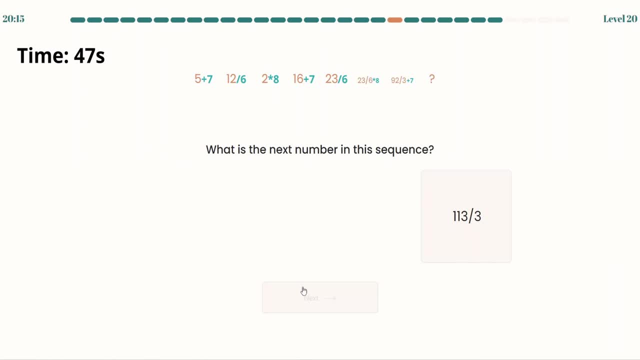 is one hundred and thirteen, So one hundred and thirteen divided by three. As you're seeing, the answer five is correct. Which figure should replace the question mark? This is another puzzle that I think is just way too hard. I spent five minutes trying to solve it. 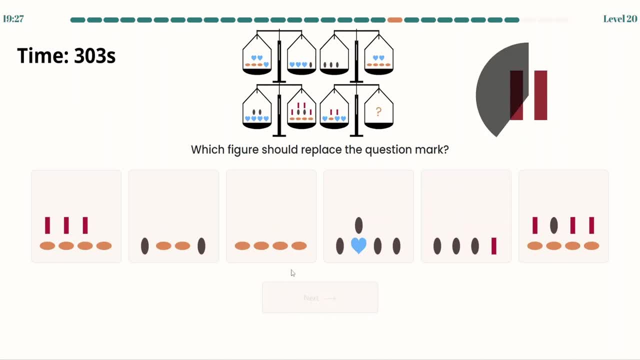 and I still answered wrong. The easiest way I have found to solve it is by first looking at the first scale and removing the three hearts on both sides, then looking at the third scale and removing the two brown ovals and dividing both sides by four to get that one heart is equal to one red line plus one yellow. 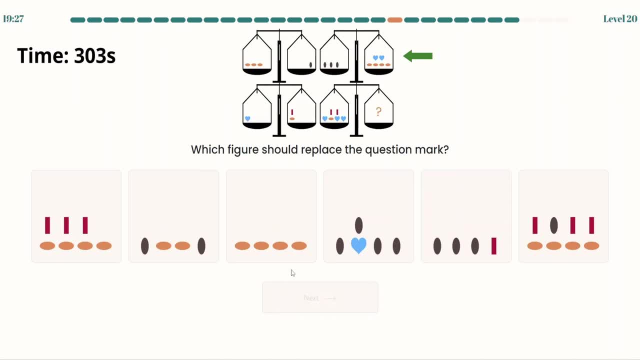 oval. In the left side of the second scale, we convert two of the brown ovals into six yellow ovals and then eliminate four yellow ovals on both sides. Now, in the left side of the fourth scale, we can convert two hearts into one brown oval and two yellow ovals and convert one. 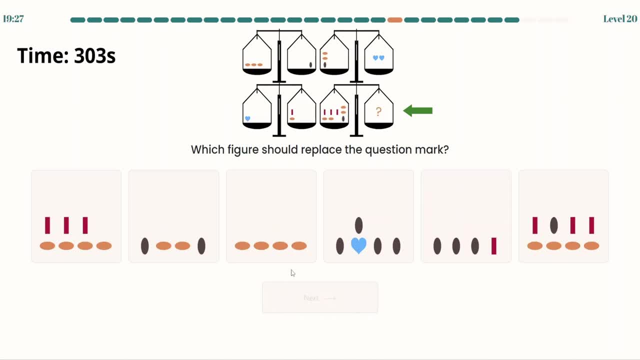 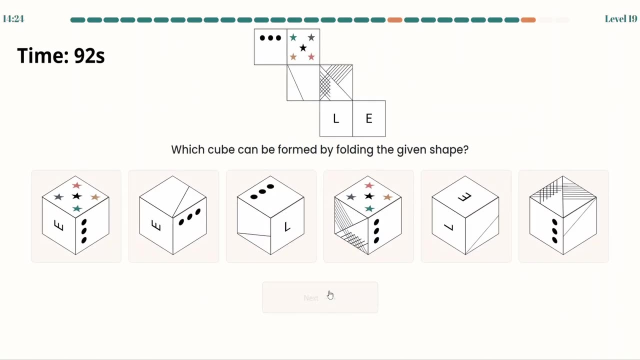 1 heart. based on the third scale into 1 yellow oval and 1 red line. These shapes so 3 red lines, 4 yellow ovals and 1 brown oval is equivalent to answer 6.. Answer 6 is correct. 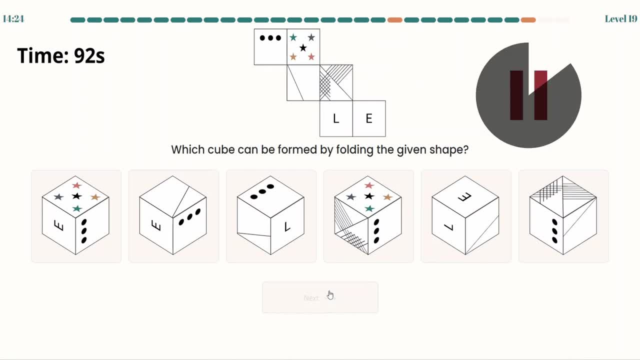 Which cube can be formed by folding the given shape, Just like the other cube forming puzzles. I will explain it by a 3D animation and not by words. So by rotating this 3D shape through a specific angle, we see that it matches answer 1.. 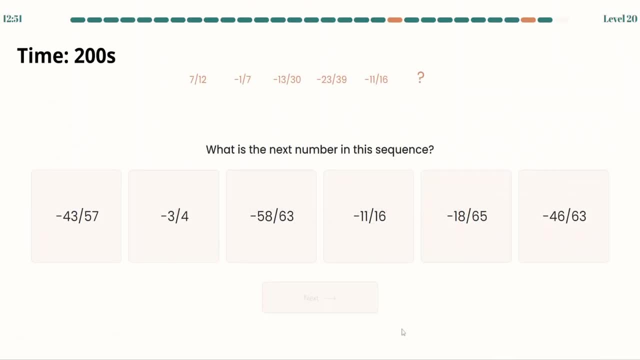 Answer 1 is correct. What is the next number in this sequence? 7 over 12, minus 1 over 7, minus 13 over 30, minus 23 over 39, minus 11 over 16?? When I took the test, I was not able to solve this IQ puzzle and I think this might be. 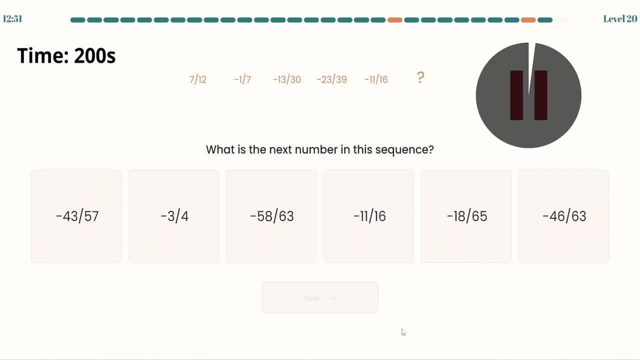 the hardest IQ puzzle that I've ever seen. So to go from 7 over 12 to minus 1 over 7,, we subtract minus 61 over 84, and then to go from minus 1 over 7 to minus 13 over 30,, we take minus 61 divided by 210.. 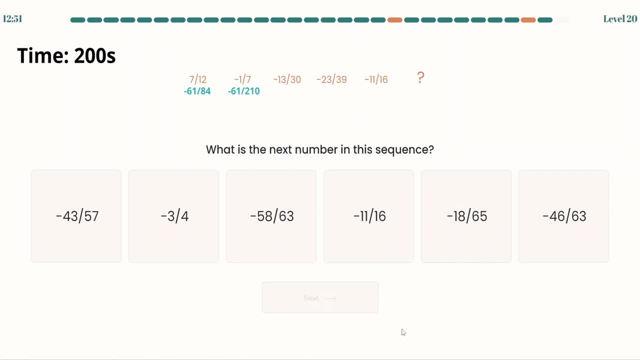 To go from minus 13 over 30 to minus 23 over 39,. we subtract minus 61 over 390. And of course nothing in total. So the answer is correct. Answer 6 is correct. Answer 6 is correct. 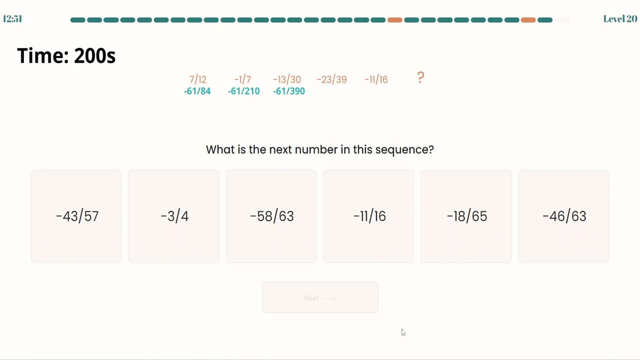 Answer 7 is correct. to go from minus 23 over 39 to minus 11 over 16,, we subtract minus 61 over 624.. Finally, to go from minus 11 over 16 to the answer, we take minus 61 over 912.. Now if we look at the numbers that we 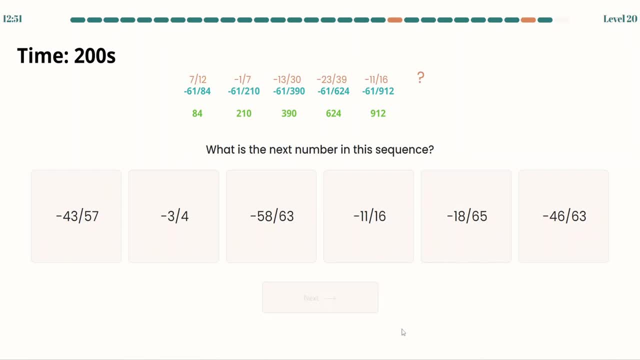 subtract. we have this predictable sequence. So if we have 84 and we add 126, then we get 210.. To go from 210 to 390, we have to add 126 plus 54. And then to go from 390 to 624,. 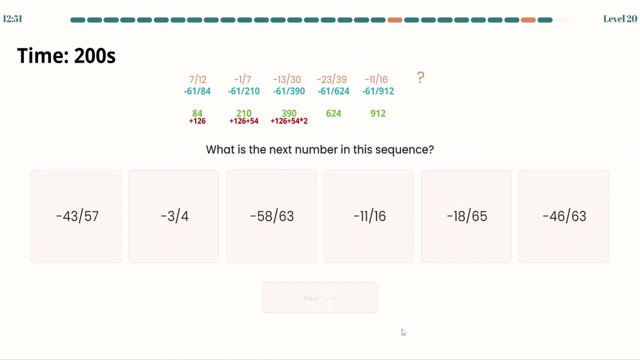 we take plus 126, plus 52 times 2. And then to go from 624 to 912, we add 126 to 912.. And then to go from 624 to 912, we add 126 to 912.. And then to go from: 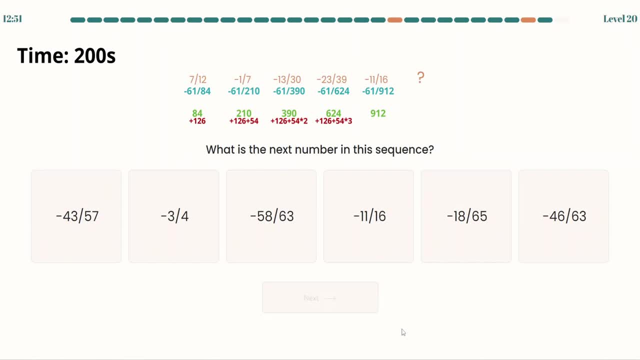 126 to 912, we add 126 to 912.. And then to go from 624 to 912, we add 126 to 912.. And then to go from 126 to 912, we add 126 plus 54 times 3.. This is absolutely insane, that you're supposed to only 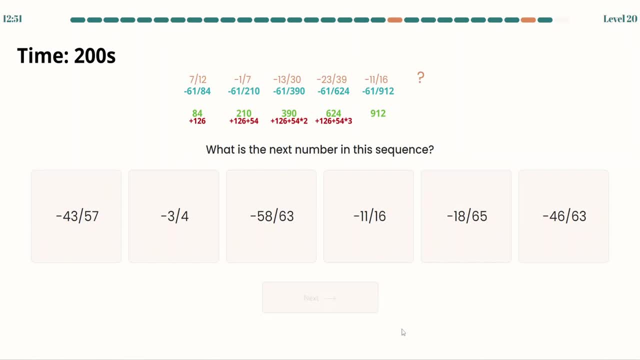 use your head to calculate these values. To show you further how complicated this gets. to find the answer, we take minus 11 over 16, minus 61 over 912.. To get the same value in the denominators, we add the top and the bottom of the first fraction by 912, and the top and 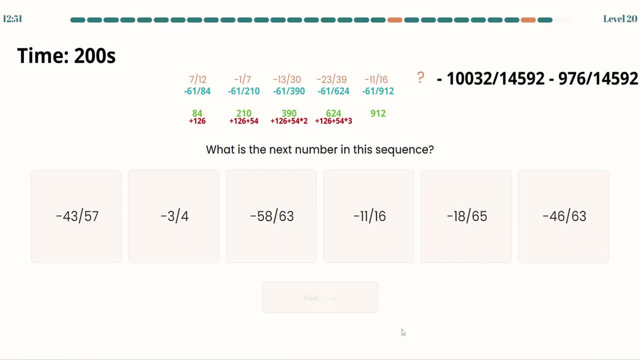 the bottom of the second fraction by 16.. This gives minus 10,032 divided by 14,592, minus 976 divided by 14,592.. We have the same denominators so we can bring them together. And now we can add: 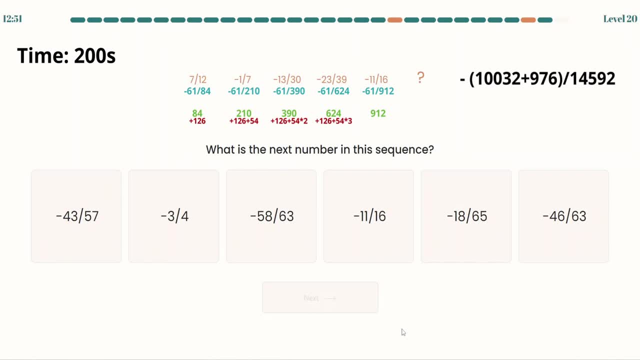 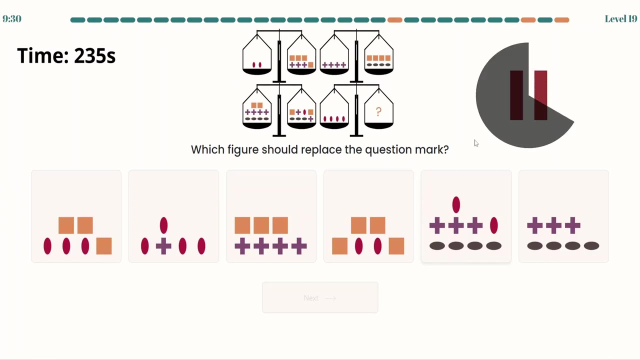 10,032 with 976 to get 11,008.. Simplifying this fraction we get, of course, minus 43 over 57.. Answer 1 is correct. Which figure should replace the question mark? I think the most efficient way to solve it is by first looking at the second scale and dividing. 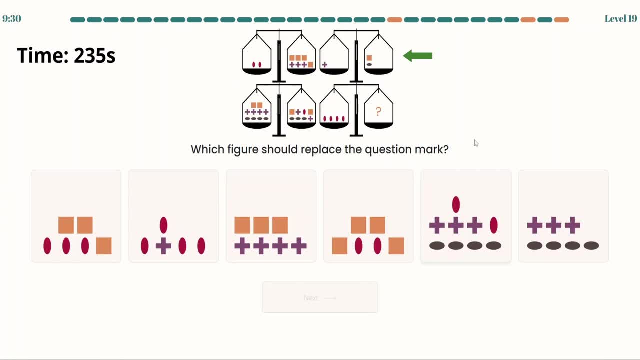 both sides by 4 to get that 1 plus sign is equal to 1 square plus 1 black oval. In the third scale we can simplify it by first removing 2 squares, then 2 plus signs and then 3 black ovals. 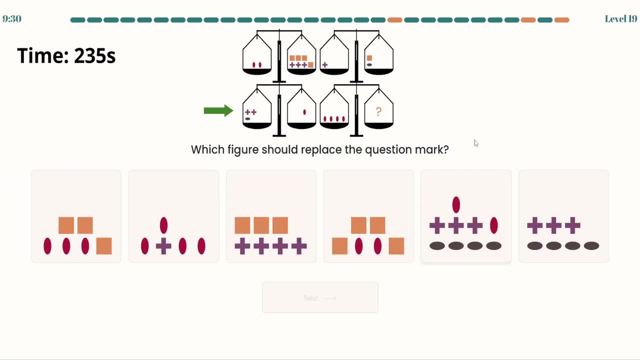 We now have that 1 red oval equals 2 plus signs plus 1 black oval. We can convert 2 red ovals on the left side of the fourth scale into 4 plus signs plus 2 black ovals. Next we can convert: 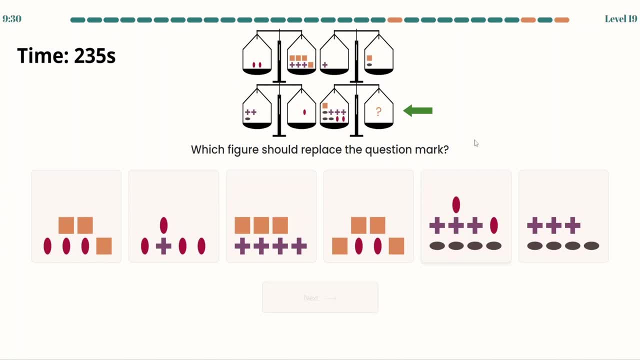 one of the plus signs into a yellow square and a black oval. Now I want to prove that the yellow squares and the black ovals have the same value. Now, by multiplying both sides of the third scale by 2, we get a 4 plus sign. We now have that 1 plus sign equals 2 plus black oval. And now we can. 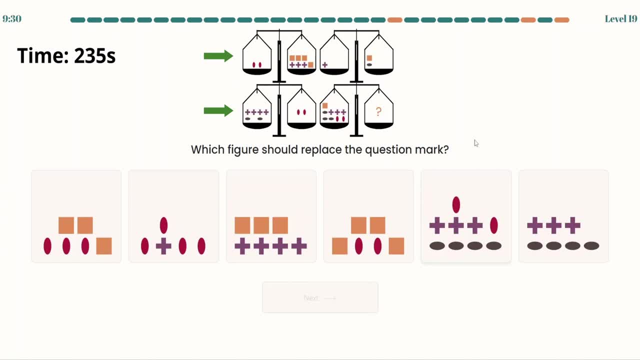 We get that two red ovals equals four plus signs, plus two black ovals. Since the left side of the first scale is equal to the right side of the third scale, we can put the left side of the third scale against the right side of the first scale. 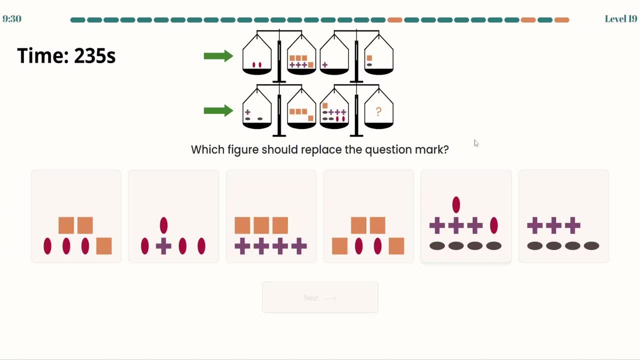 Now we can eliminate three plus signs on both sides and the remaining plus sign we can convert into a yellow square and a black oval. By removing one yellow square on both sides and dividing both sides by three, we see that one yellow square equals one black oval. 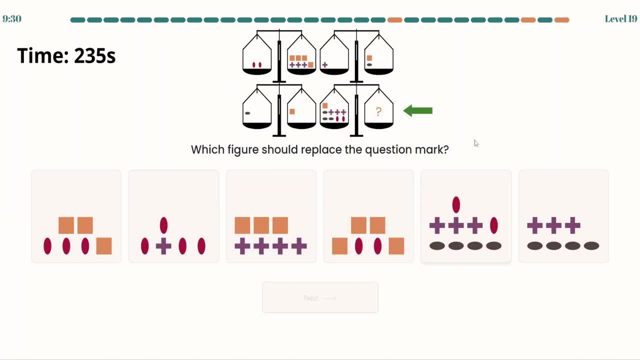 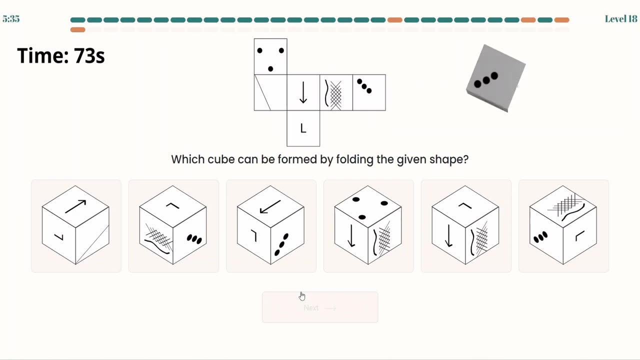 The yellow square on the left side of the fourth scale we can convert into a black oval. The left side is now equivalent to answer five. Answer five is correct. Which cube can be formed by folding the given shape? Again, one of these cube folding puzzles that. 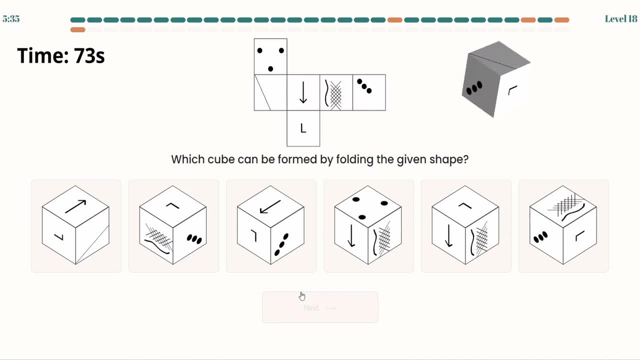 are hard to understand. So I created this 3D model and by looking at the 3D model from a specific side, we can see that it matches answer four. Answer four is correct. What is the next number in this sequence? 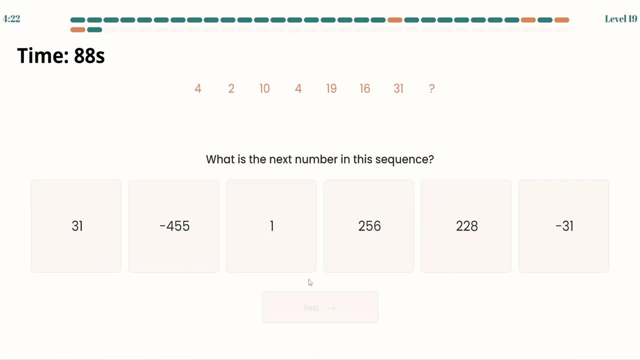 Four, two, ten, four, nineteen, sixteen, thirty one question mark. First let's pull down every odd number, element Four, ten, nineteen, thirty one. Four plus six is ten, ten plus nine is nineteen, and nineteen plus twelve is thirty nine. So we just increase by three every time we add. 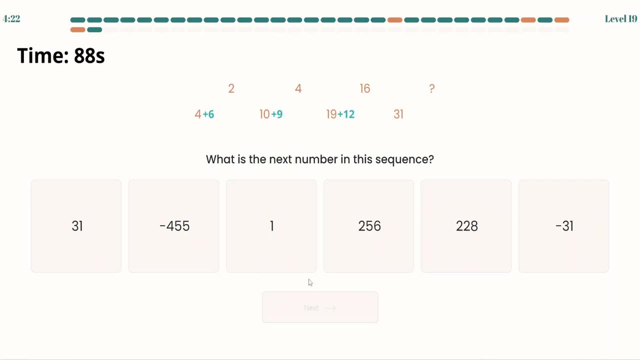 On the top we have two, four, sixteen question mark. Two squared is four. four squared is sixteen. sixteen squared is two hundred and fifty-six. Answer four is correct. This was the last puzzle that I answered during the test. Which figure should replace the question mark?